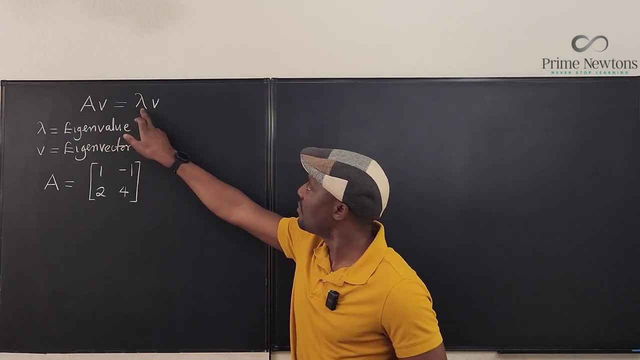 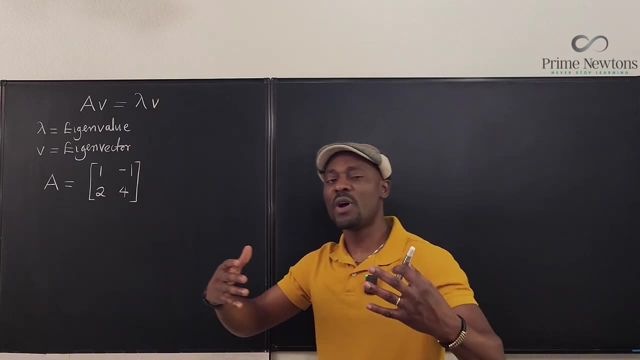 A is a matrix, v is a vector, but Lambda is a scalar. it's just a number and this is a vector. Let's see if you were able to guess how important it is to know this. we want to try and solve an equation. watch what's going to happen. We're going to say: 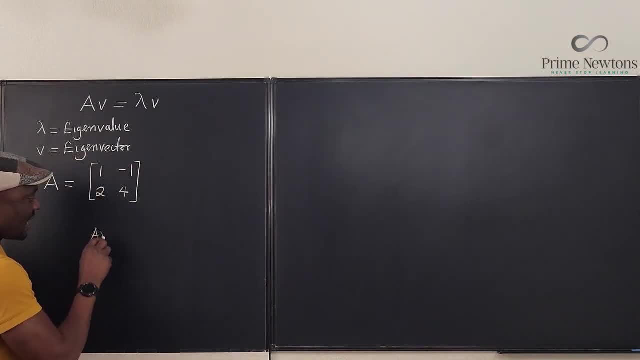 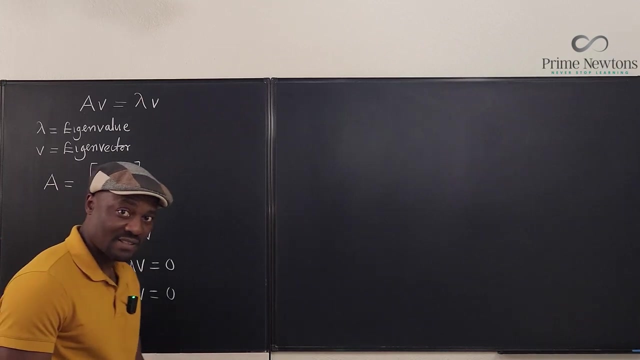 that a v equals lambda v. Let's move everything to one side. We've got a v minus lambda v equals zero. Now watch this. Let's factor out the v: a minus lambda times v is equal to zero. Now this looks fantastic, but it's meaningless. It is stupid. Why is it stupid? Because you cannot. 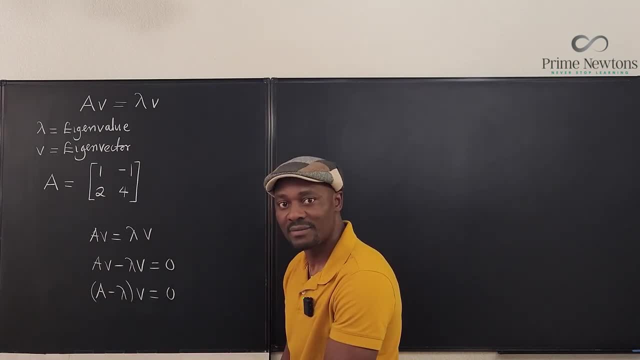 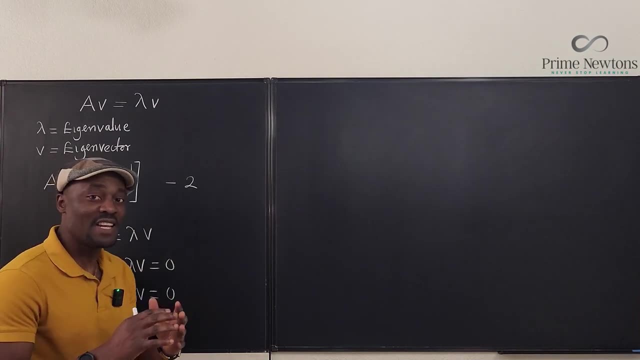 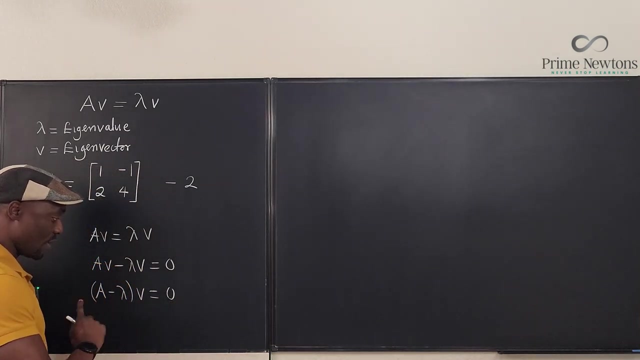 subtract a number from a matrix. No, this is what a matrix looks like. So it's like saying this minus two. See, you cannot subtract anything from a matrix unless the other thing is also a matrix. So we cannot work with this. The only way we can work with this is if we make this. 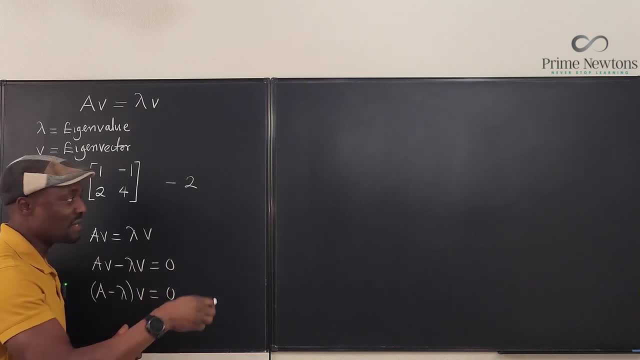 also a matrix. So we cannot work with this. The only way we can work with this is if we make this also a matrix And there's a quick manipulation we can make. What if we multiply it by the one of matrices? The one of matrices is the identity matrix. Remember, it is that matrix that just has. 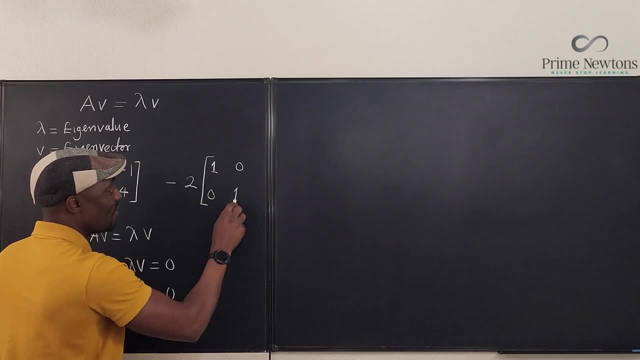 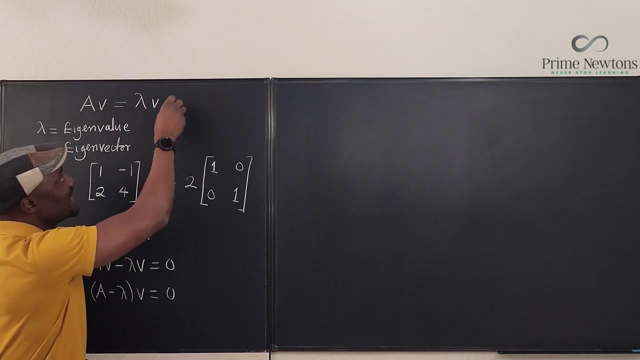 one here has zero here has zero here, has one here. Now, when you multiply this by this, you have put the two in the correct positions. So this actually is a good manipulation. So we can go back to this original equation and say that this is equivalent- let me just put it this way- to a v is equal to 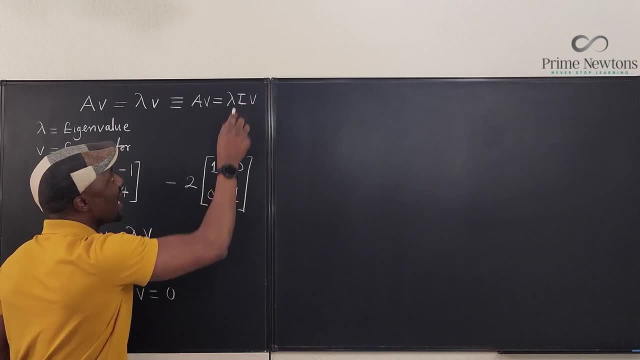 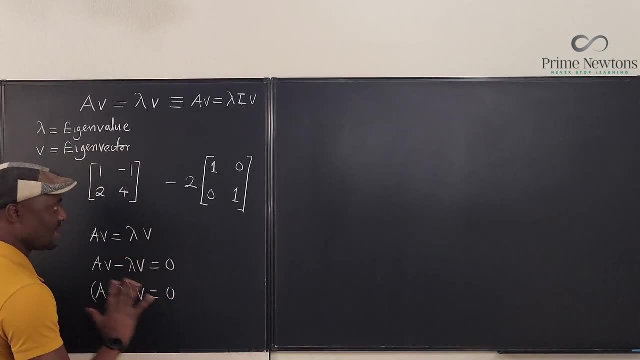 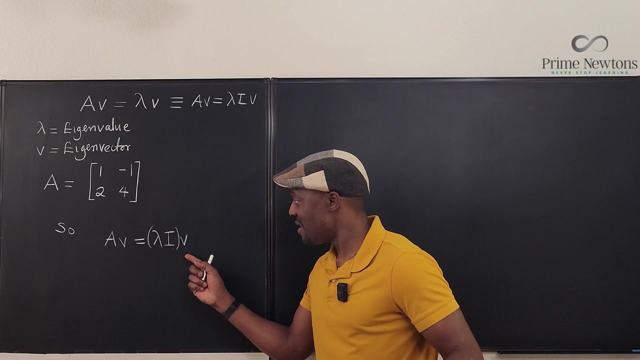 lambda i v. You see this, i doesn't change anything in matrices because it's the identity. It's like multiplying something by one. So instead of us using this equation that I wrote here, this is what we're going to use so we can do this subtraction. So now we've got a v equals lambda i. 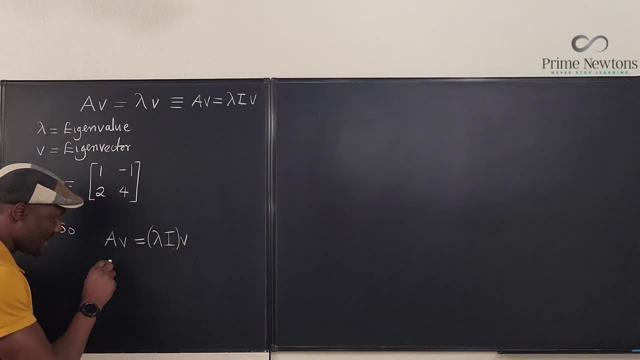 v. Let's continue. So we're going to have: we're going to say that a v minus lambda i v equals zero. We can factor out the v and say: a minus lambda i times v is equal to zero. Okay, Now you know how we can actually. 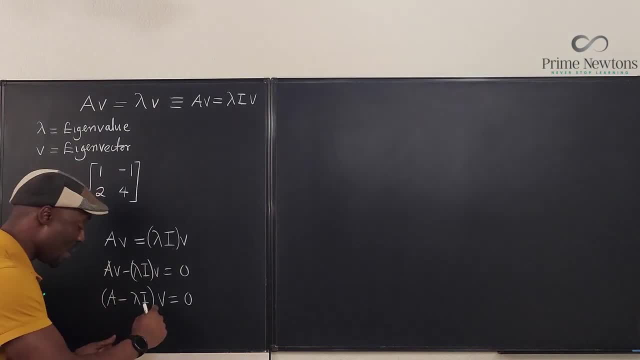 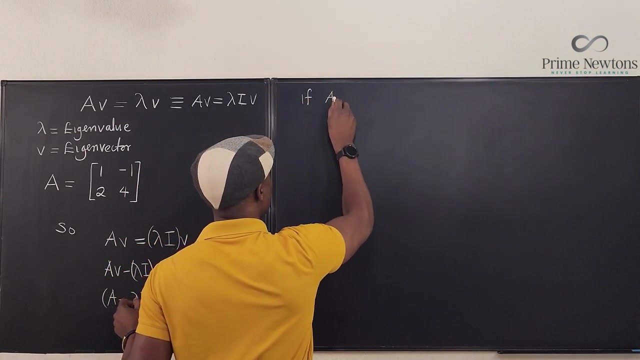 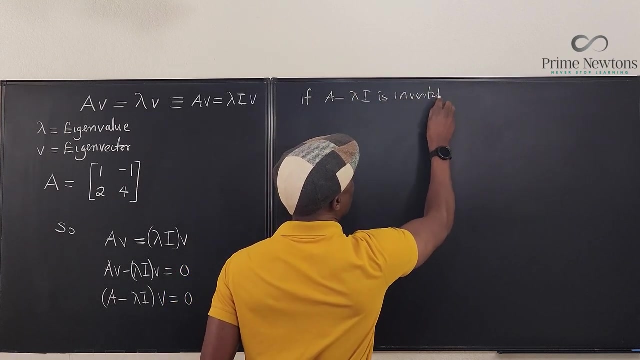 get our v, Because if we get our v, all we have to do is find the inverse of this matrix and use it to divide zero. But if we're able to do that, so look if a minus lambda i is invertible. if we can find the inverse of this, then what we can do is we're going to use the. 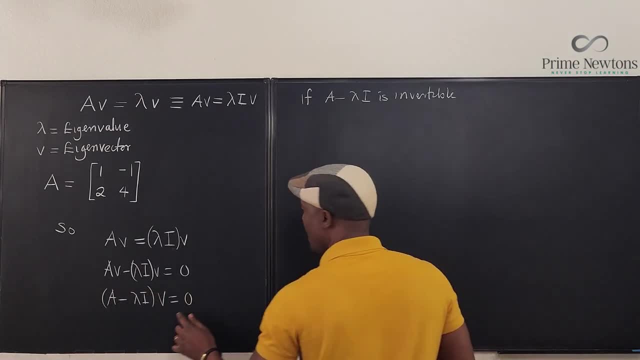 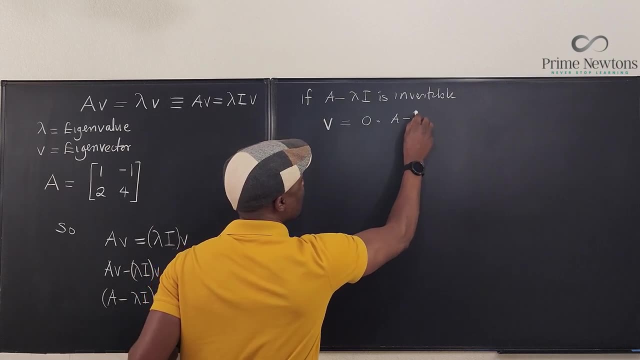 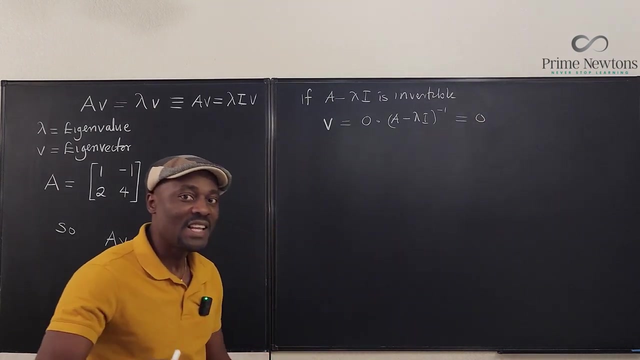 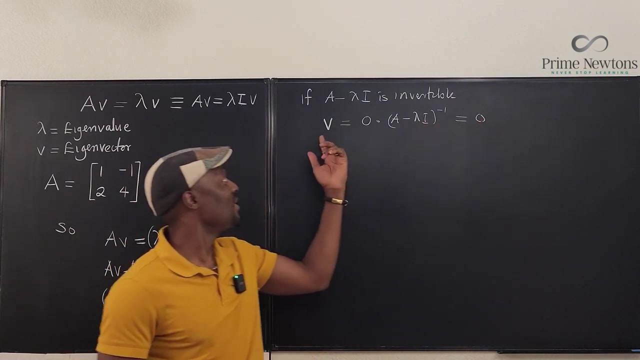 inverse of this, to multiply this side and multiply this side, And we're going to end up with v, will be equal to zero times a minus lambda. i inverse, And what would this be? This would be equal to zero. But the eigenvector of any matrix can never be the zero matrix, So you can't have the zero matrix as an 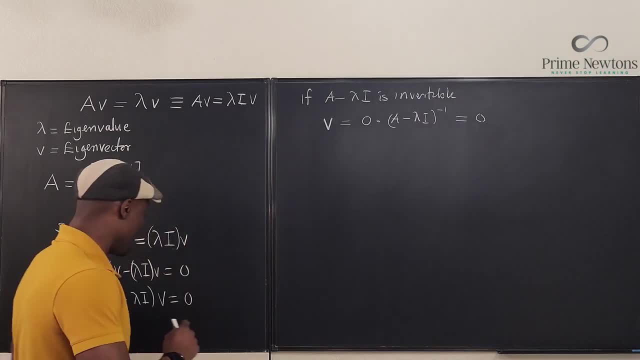 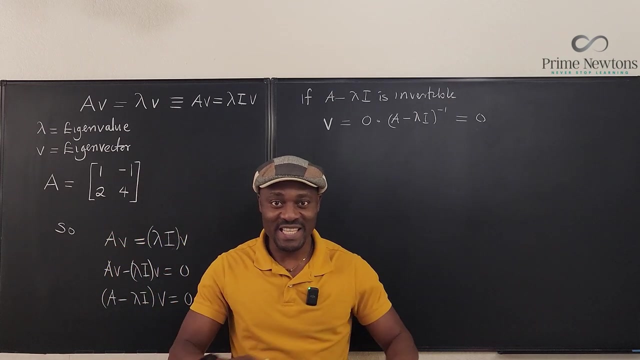 eigenvector. So the only way what we just did is meaningful is if this is not invertible. if this is not invertible, then the determinant of this matrix is equal to zero, And that is our key to finding the eigenvector and the eigenvalue. So, since this, 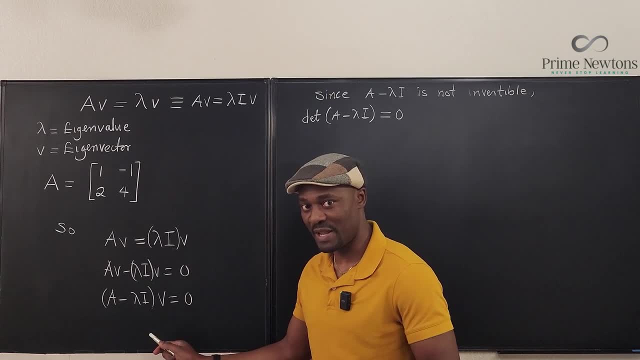 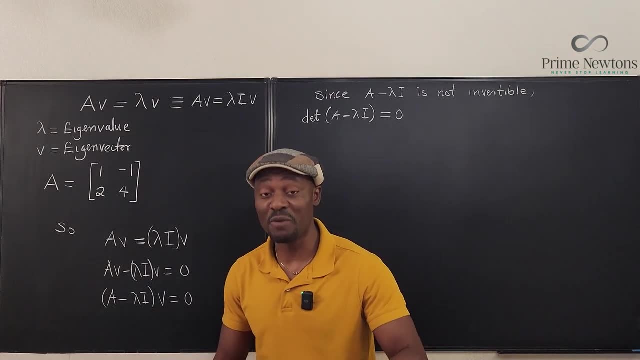 is not invertible. okay, I already explained why, then. the determinant of this matrix is zero. That's the meaning of not invertible. The determinant of a matrix is equal to zero if the matrix is not invertible. Or a matrix is not invertible if the determinant is equal to zero. 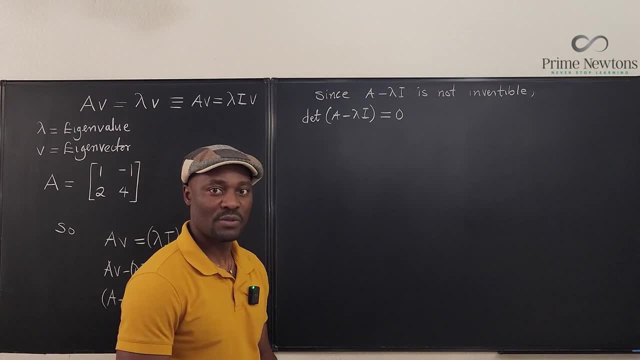 So we know that the matrix is not invertible. So we know that the matrix is not invertible, So we know that the determinant of this matrix is equal to zero, And that's it. So let's begin our calculation to find what this is going to be. So look, this is what you're going to have. 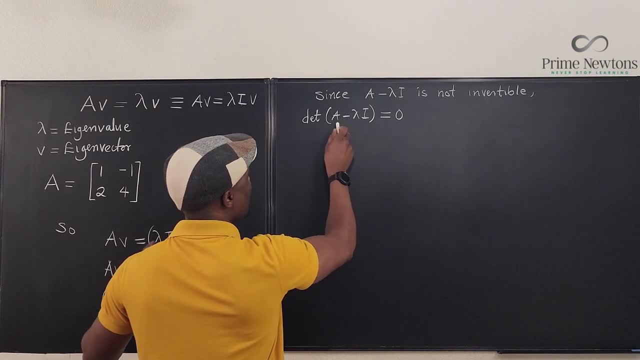 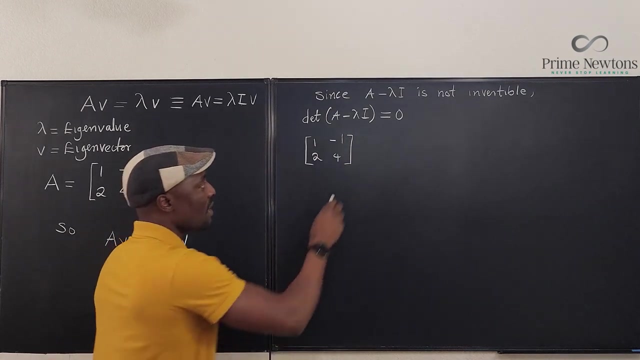 You're going to have the determinant of: firstly, let's find a minus delta, a minus lambda i. So a, what is a? So we have this matrix. It's going to be one minus one, two, four Minus lambda. 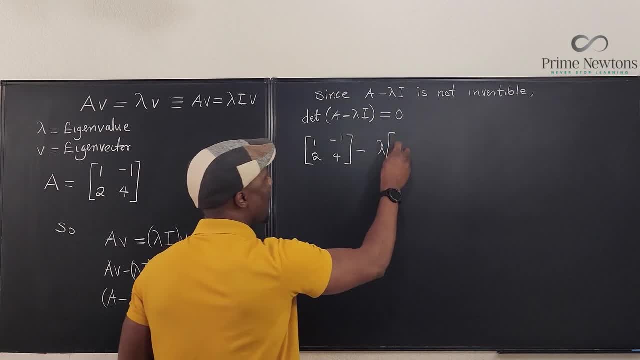 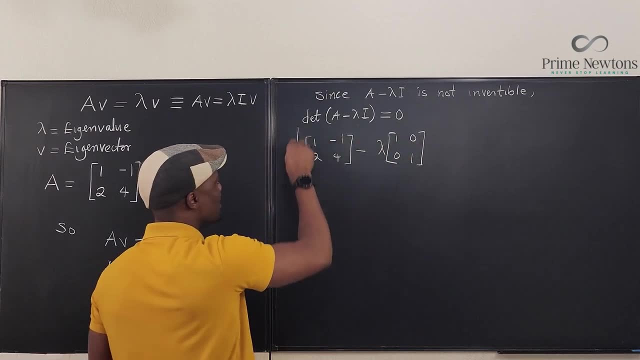 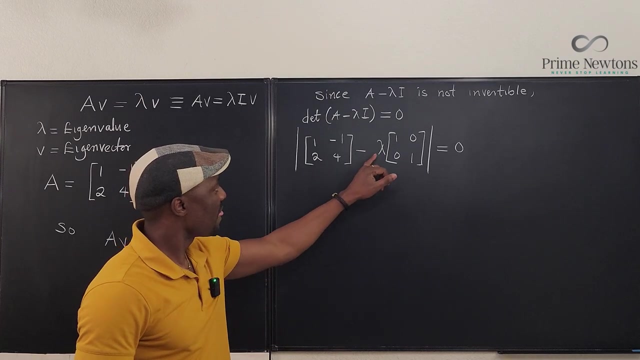 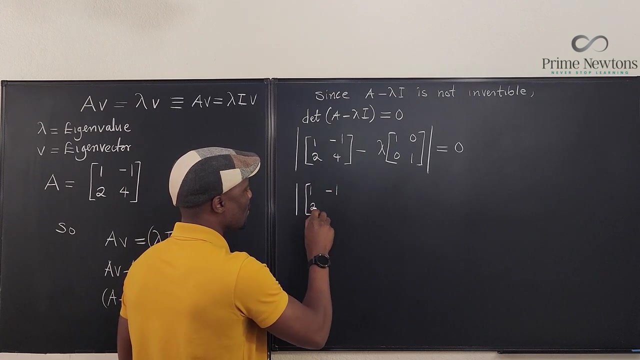 Times. i. What is i? i is one, zero, zero one. We're saying that this is going to have a determinant that is equal to zero. Okay, Well, this is the determinant of one. Let's put this together: Minus one, two, four, Minus- this is lambda. 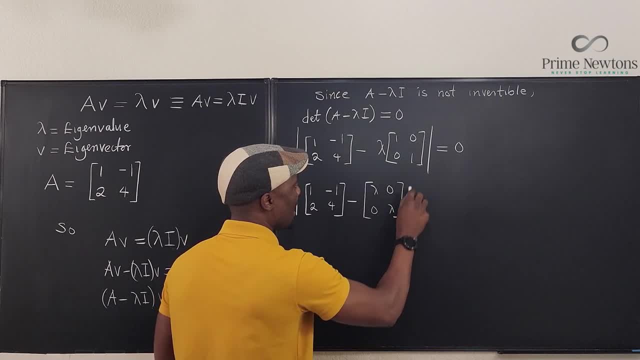 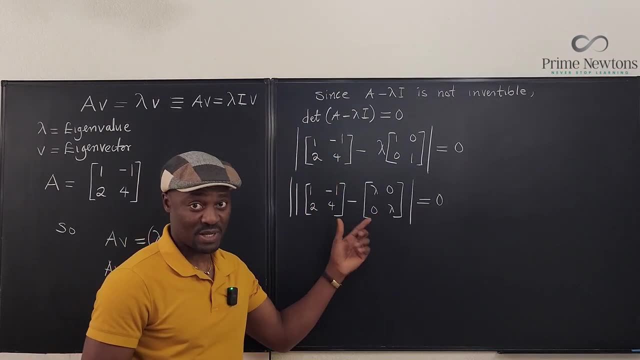 Zero, zero, lambda. Okay, The determinant of this is going to be equal to zero. Well, you can subtract this matrices now, because they have the same dimension. Remember, you can only subtract when the dimensions are the same. So we're going to subtract and you subtract corresponding entries. 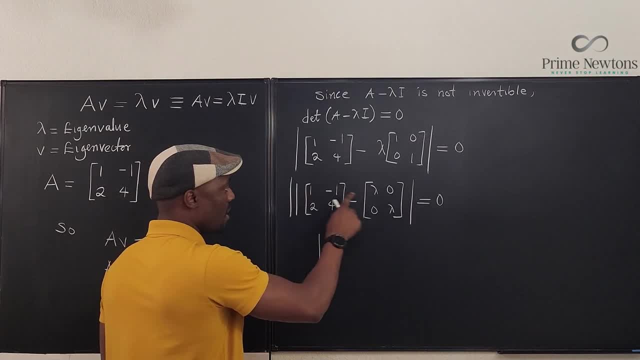 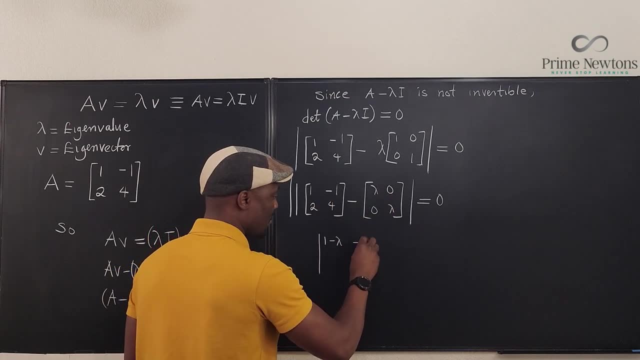 So the determinant of this matrix, one minus lambda, is the first entry here, And here it's going to be negative. one minus zero is just minus one, And this is going to be two minus zero, That's two, And this is four minus lambda, That's four. 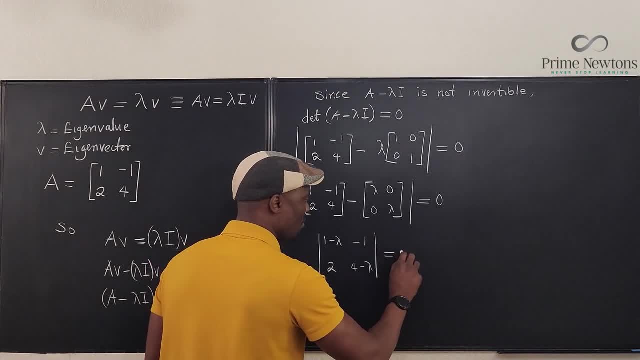 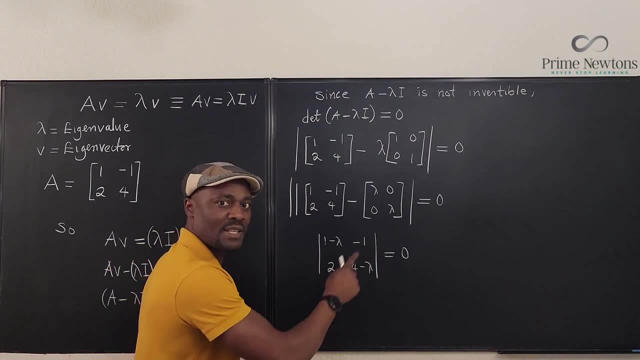 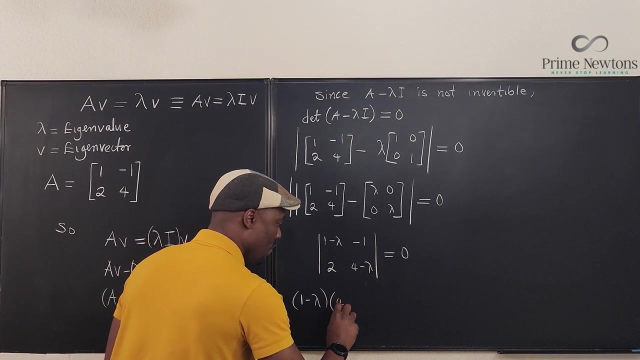 minus lambda, So this determinant has to be equal to zero. How do you compute the determinant of a matrix again? Well, you multiply these two entries and subtract these two. So let's do it. So it's going to be this times this, which is one minus lambda, times four minus lambda, minus two times. 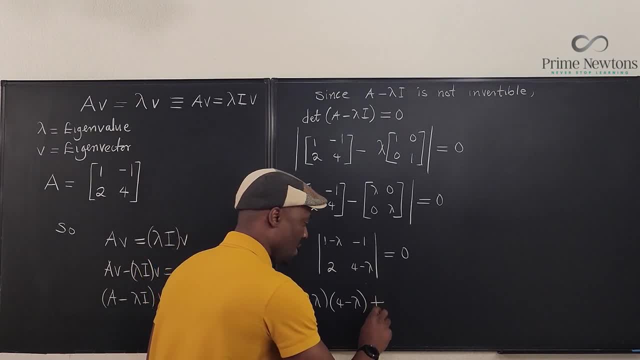 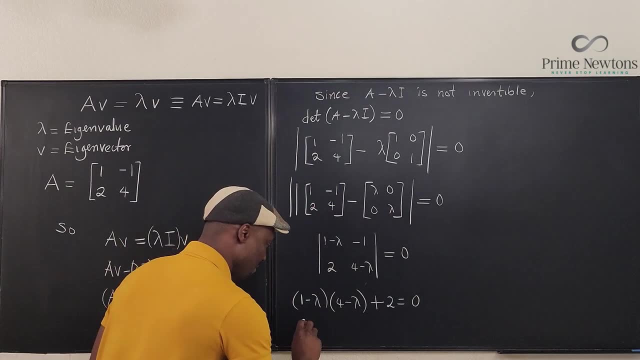 minus one, That's going to be minus two. Minus minus two will be plus two Equals zero. Let's clean up. Can we distribute this? Yes, If you distribute this, you'll end up with lambda squared minus five. lambda plus four plus two equals zero. So see what we've got. 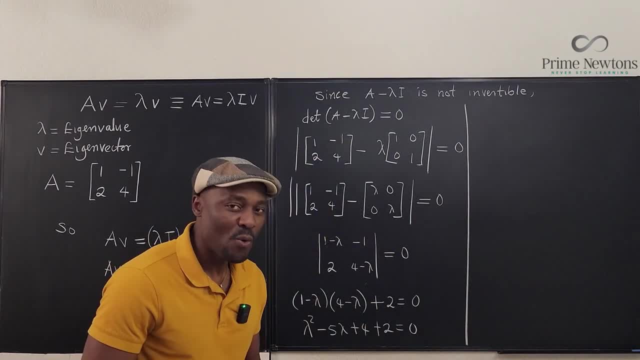 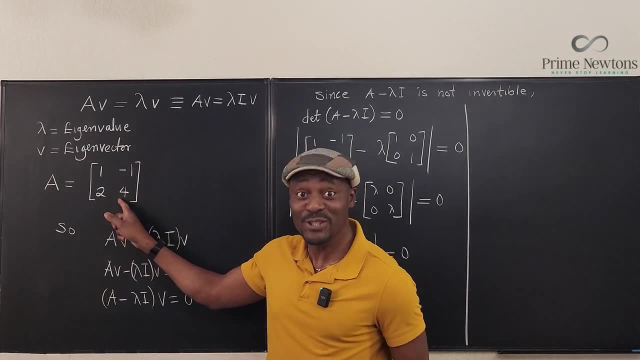 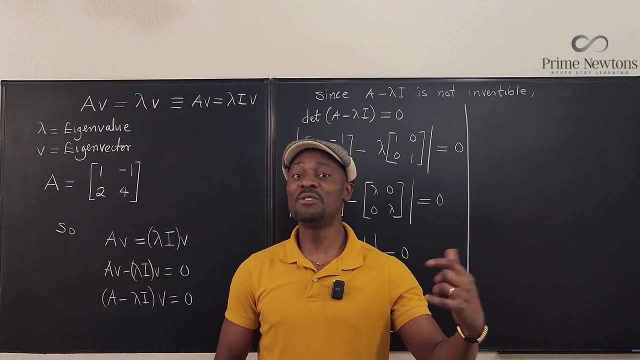 We're going to end up with a quadratic equation. Why would it be quadratic? Well, it's going to be a polynomial of degree two. Why would it be of degree two? Because this is a two by two matrix. So whenever you have an n by n matrix, you're going to have a polynomial of degree n. if this, 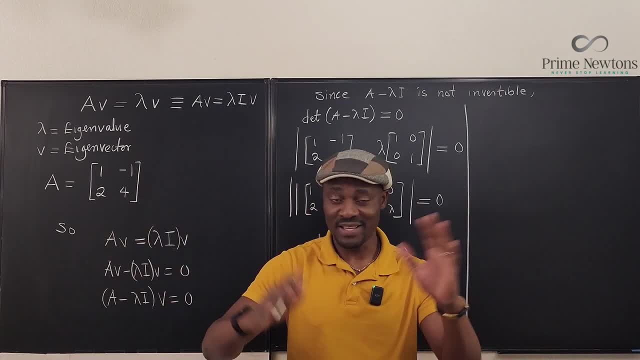 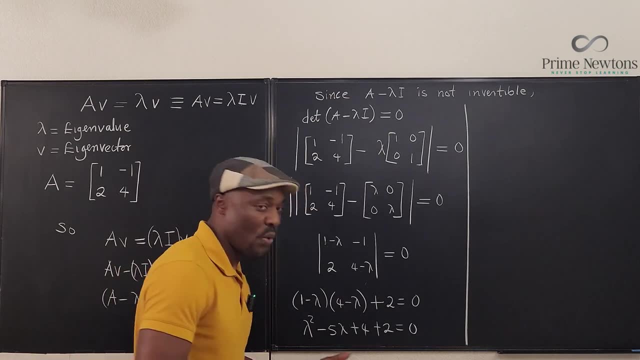 is a square matrix. Okay, We're going to talk about other things in the future, because it gets more complicated if we do more advanced linear algebra or we do numerical analysis. Now, at this point, this is what we have. If we clean this up, this is lambda squared. 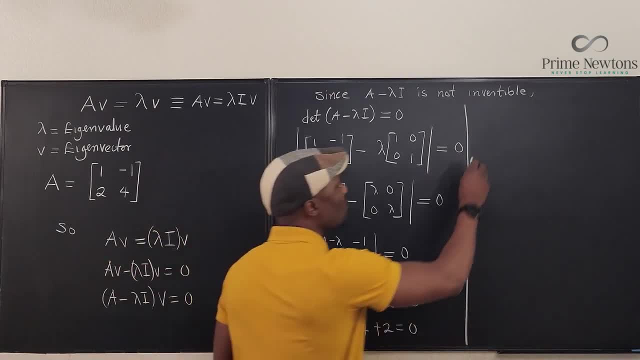 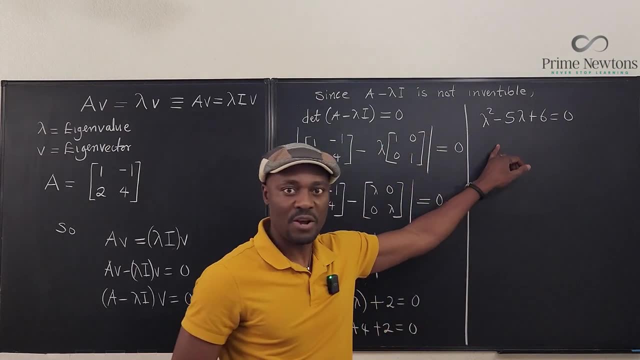 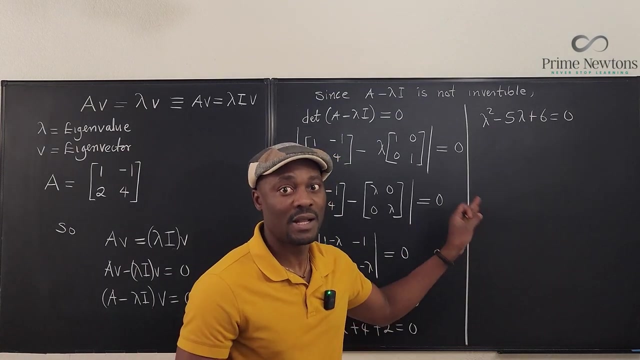 minus five lambda plus six equals zero. So we've got lambda squared minus two. 5 lambda plus 6 equals 0.. Well, this is a very common quadratic equation. We know that if we solve this, we're going to get x equals 2 or x equals 3, right Or not? x lambda, Okay. so we 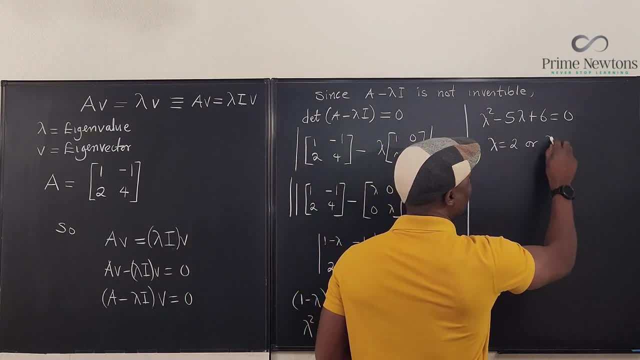 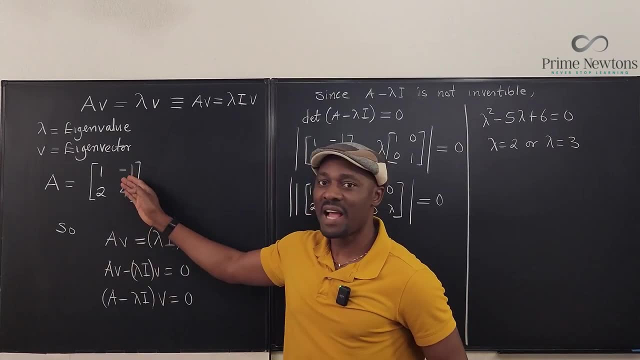 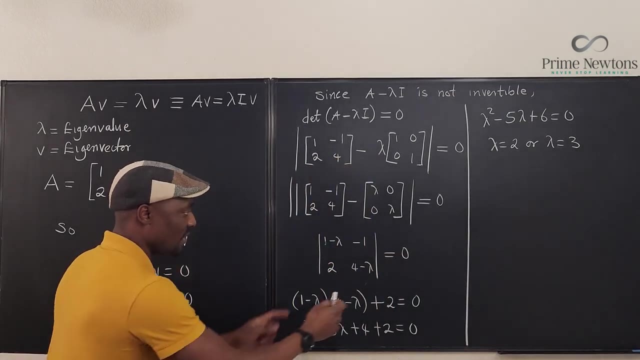 have lambda equals 2 or lambda equals 3.. These two lambdas are the eigenvalues. It is very straightforward. What I showed you at the beginning was the justification for this equation. You don't need to show any of these when you do the calculation. All you have to do is 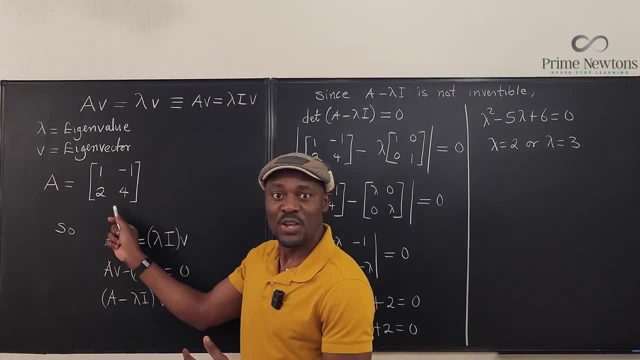 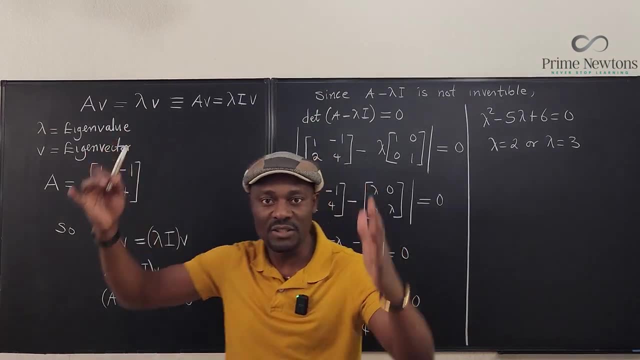 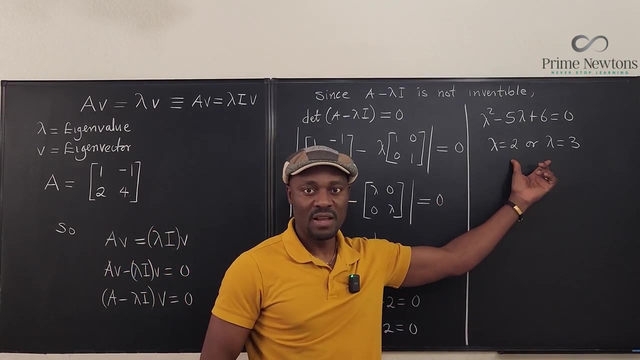 whenever they give you a matrix like this: okay, just subtract lambda from here, subtract lambda from here, That's all you need. And take the determinant of the resulting matrix, equate it to zero, solve the quadratic. you get your eigenvalues. Okay, I explained to you why. 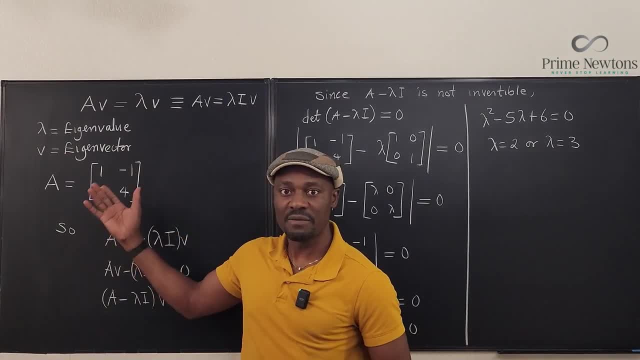 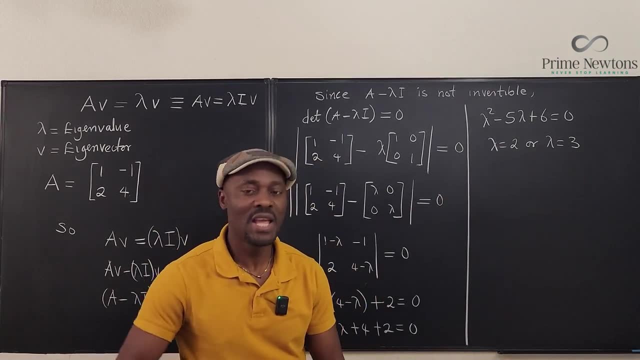 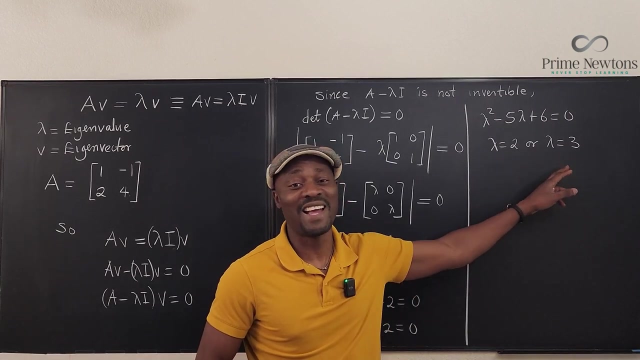 we had to do this, It's because of the theory, the definitions. That's what led us to this. So, now that we have the eigenvalues, all we need are the eigenvectors. In other videos I'm going to show you the applications and the usefulness of these guys. They save lives, I tell you okay. 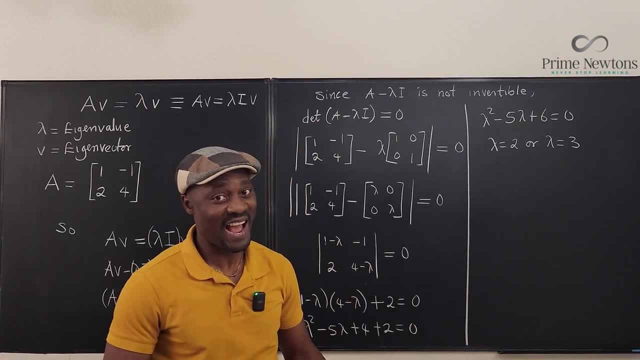 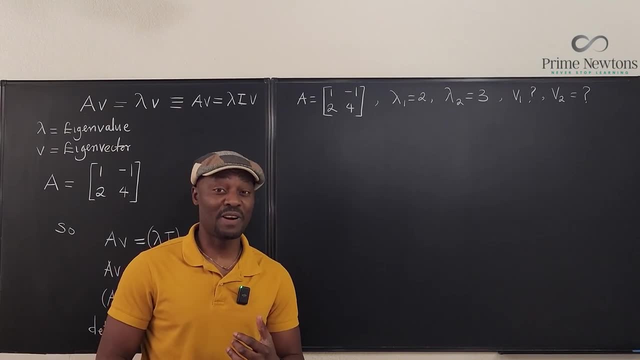 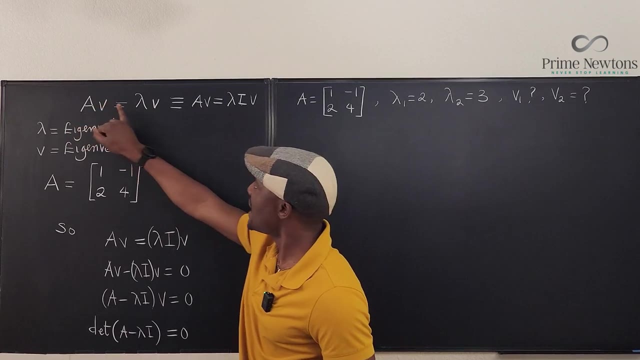 Because when the going gets tough, the eigenvalues and the eigenvectors just get going. Now we have our two eigenvalues. We need to find the eigenvalues Because, remember, this equation is not complete. We already know what A is and now we found two. 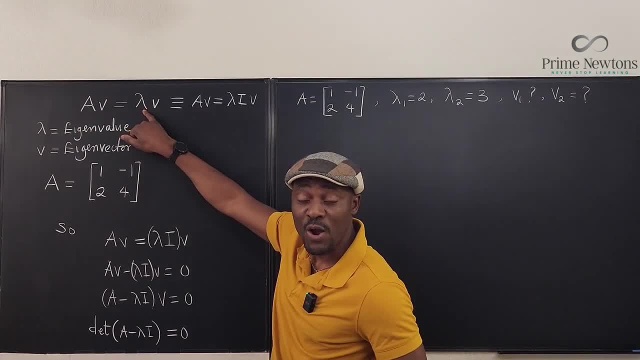 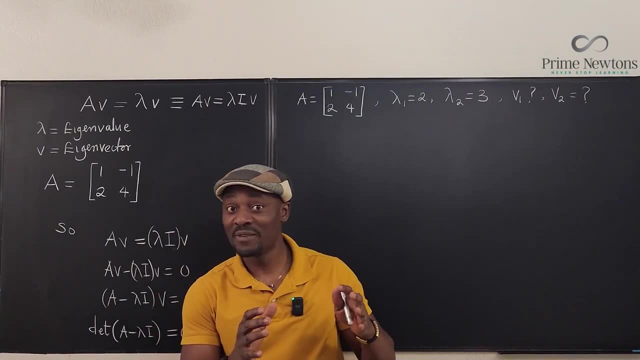 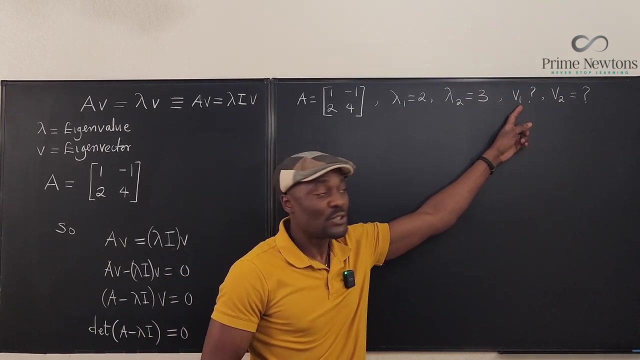 values for our eigenvalues, right? We just need to know what the eigenvector will be for each of them. So each eigenvalue has its own eigenvector. That's why I labeled them lambda one and V one. So this is going to go with this, and this is going to go with this. There are times where 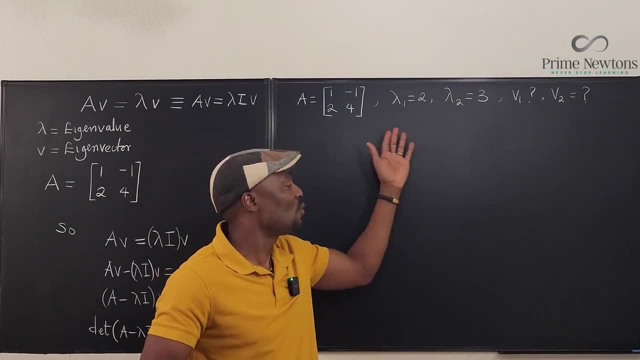 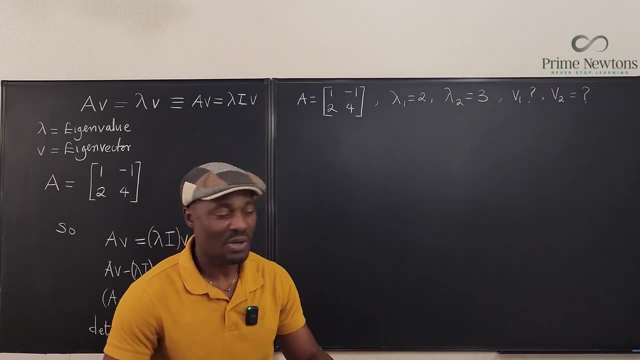 these two are the same. That's a simple equation. So now we have the eigenvalues and now we have the special situation. There are times where they share the same eigenvalue. There are times where the eigenvectors are the same. Well, those are special situations, but let's just take the normal. 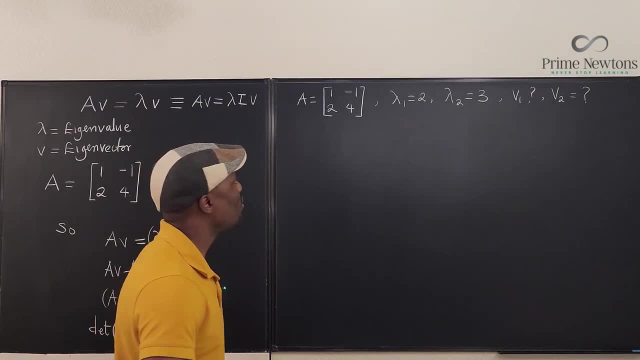 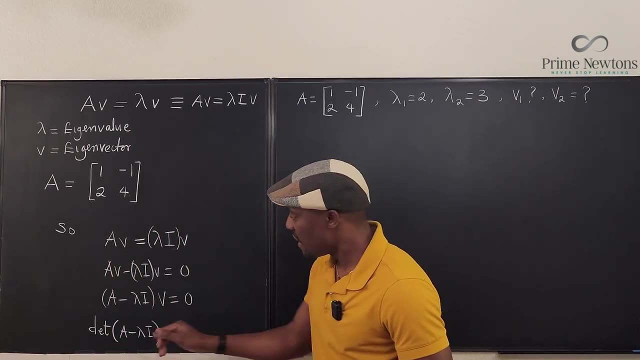 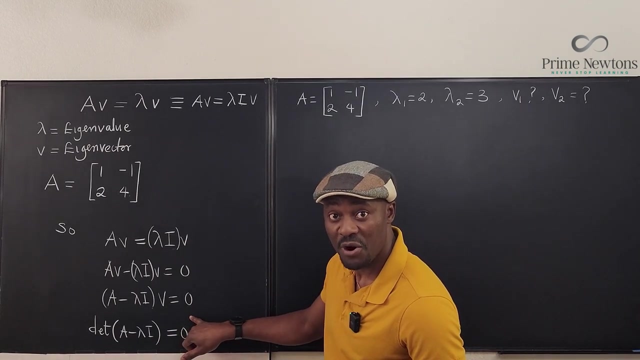 situation that is normally expected. okay, So how do we find the eigenvalues? You go back to this equation. Remember what we said: that A minus lambda I will always be multiplied by V and the answer is supposed to be zero. Yes, We don't know what V is. 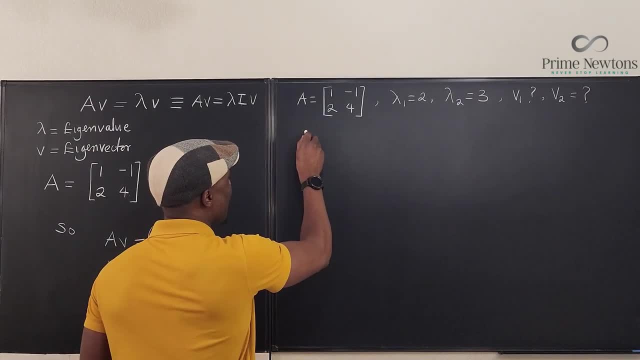 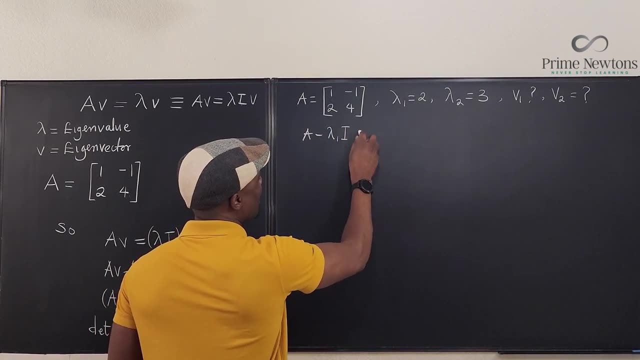 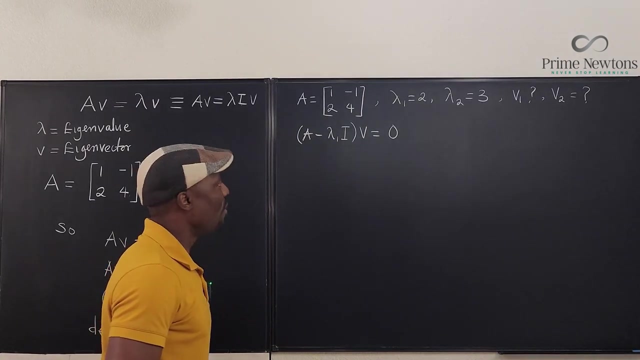 So this is the setting we're going to have. We're going to say that A minus lambda I let's do lambda one I multiplied by V will be equal to zero. So let's plug stuff in. What is A? This is: 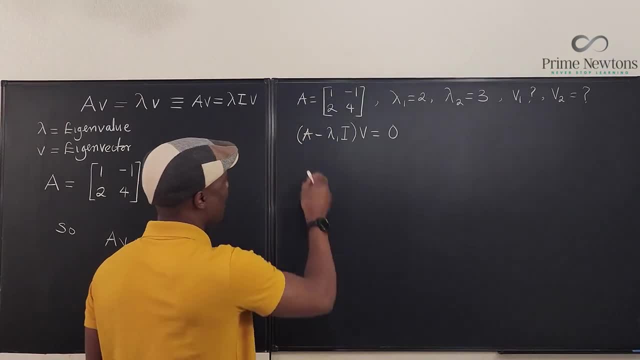 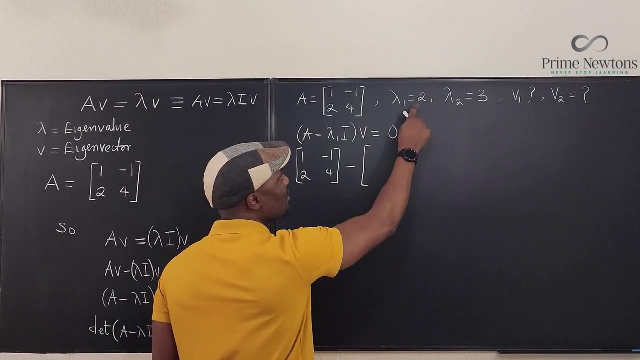 A. A is I'm going to write a lot this time, so it's going to be one minus one, two, four. This is A. We're going to be subtracting Now. you see our lambda. one is two, So two times the identity. 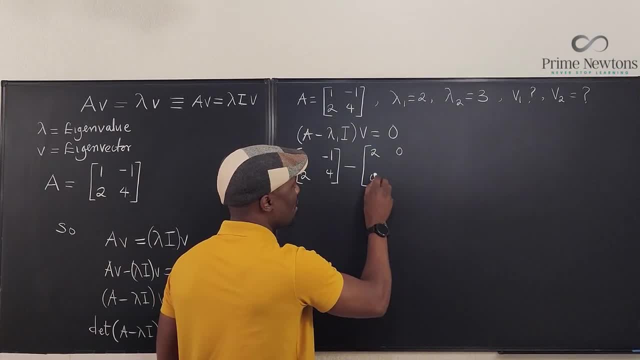 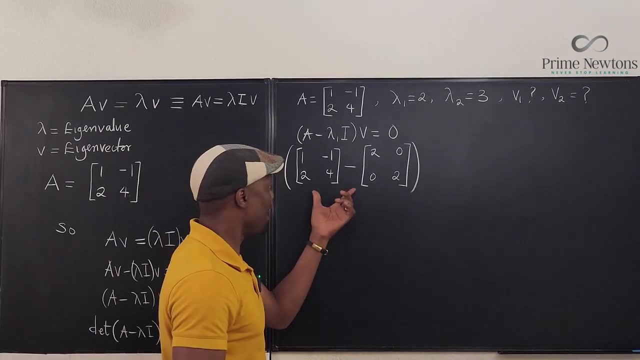 matrix is just going to be: you're going to have two here, zero two. I don't want to write the identity matrix separately anymore. So this is what you are actually subtracting, right? We're multiplying this matrix, that we're going to get by V from this formula, but we don't know what V is. 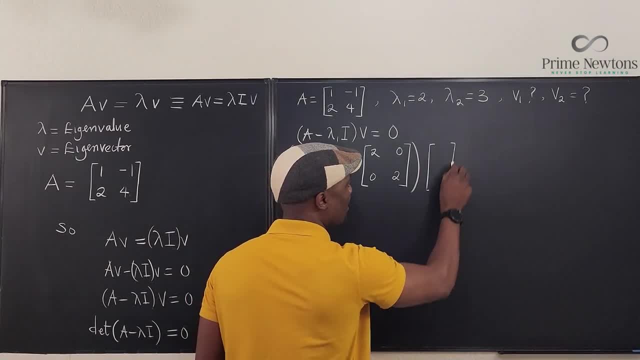 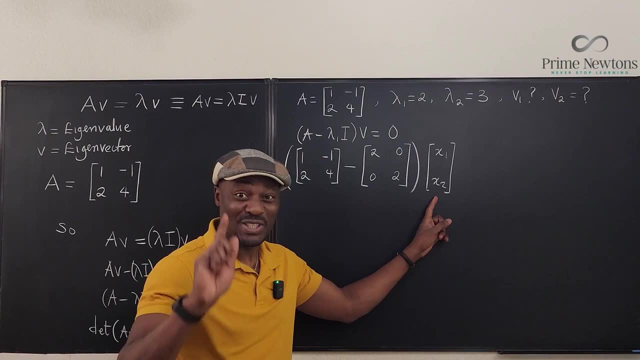 So let's just represent V as a column matrix. okay, It's usually going to be. let's call this X1, call this X2.. This is our eigenvector. We just need to know what X1 is and what X2 is and we'll be fine. okay, And on the right-hand side, 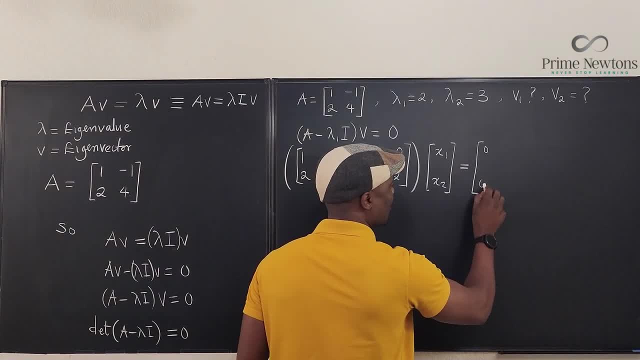 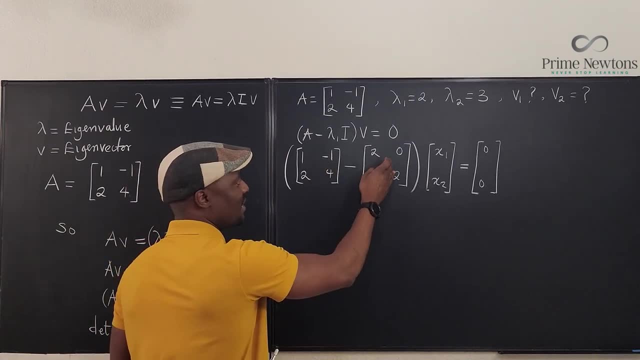 we're going to get zero. This is how to represent this as zero. okay, And that's what you have. So let's do our calculation. If you subtract this from this, it is basically you subtracting two from this and from this. Remember, that was the formula we had. 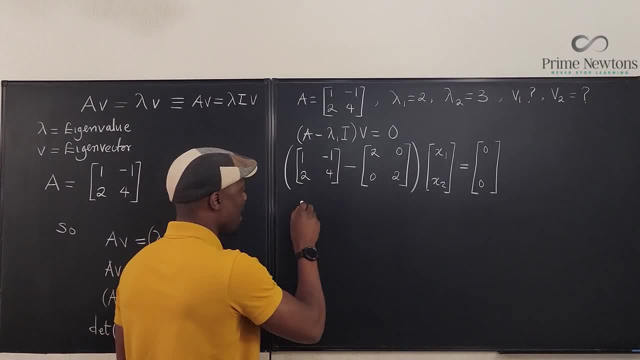 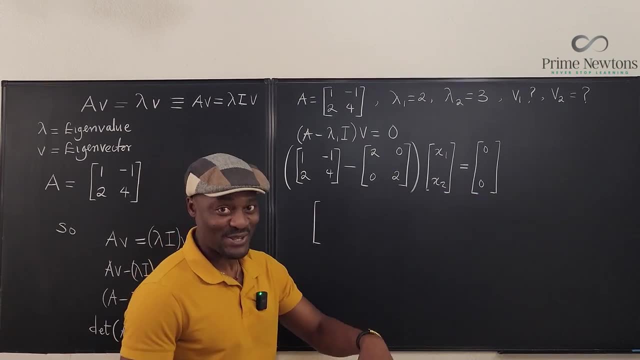 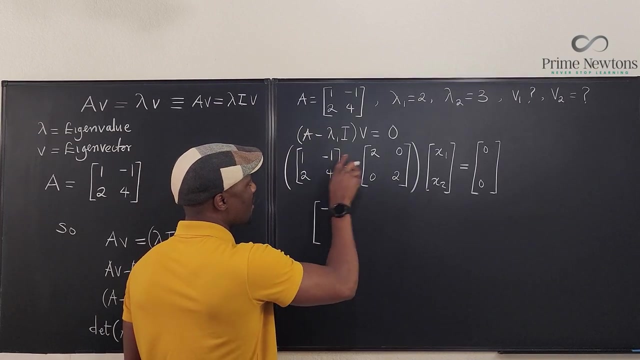 solved the equation with. So here, we're going to go here and say that this is the second time I do this. I'm not going to go through this process, I'm just justifying the shortcut I'm going to use in the second part. So this is going to be one minus two. that's going to be minus one and minus. 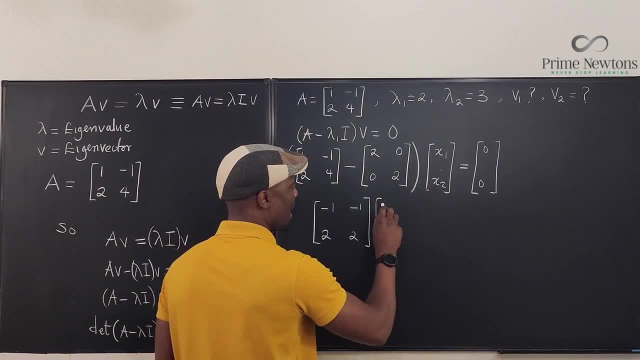 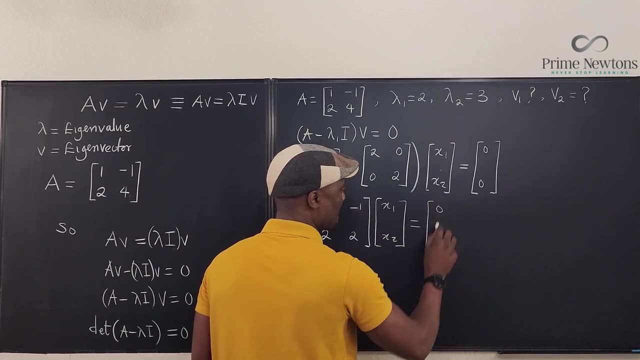 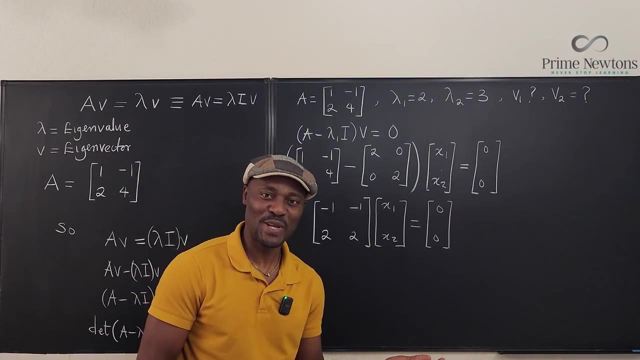 one minus zero. So I have this multiplied by X1,, X2, and what I get here is this: Okay, So now we need to solve this equation. but this is easy, This is super easy. What do we do? 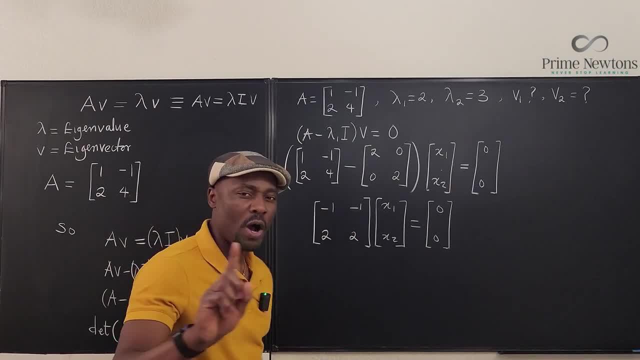 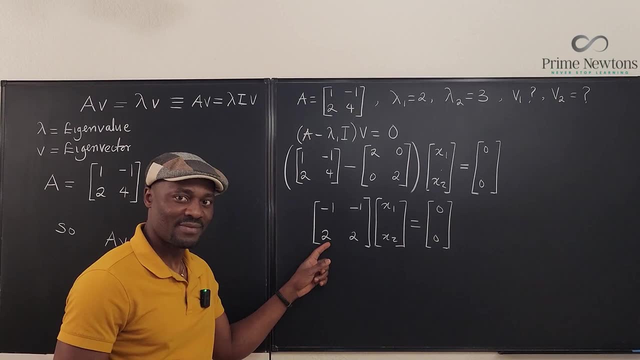 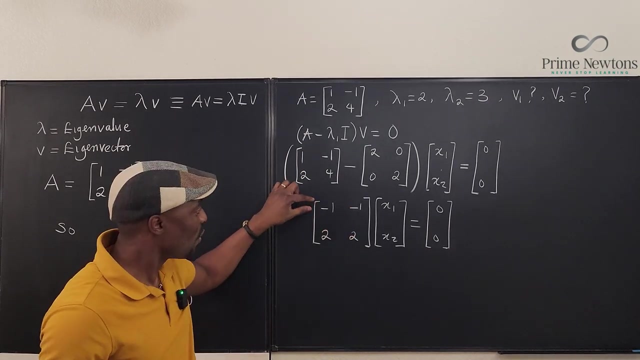 Multiply row by column. This multiplied. Oh observation, Did you notice that this is a multiple of this? right, You can just multiply this by negative two. you're going to get this. Multiply this by negative two, you get this. So if you really really want to get non-zero, 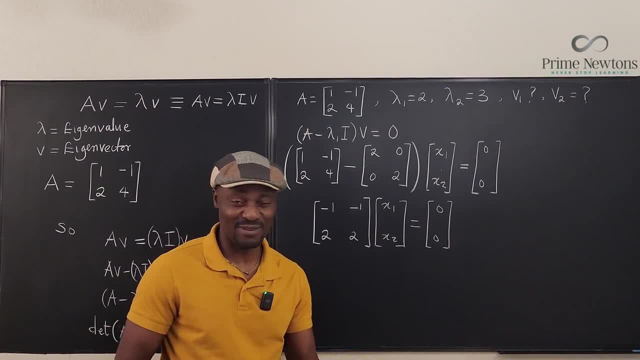 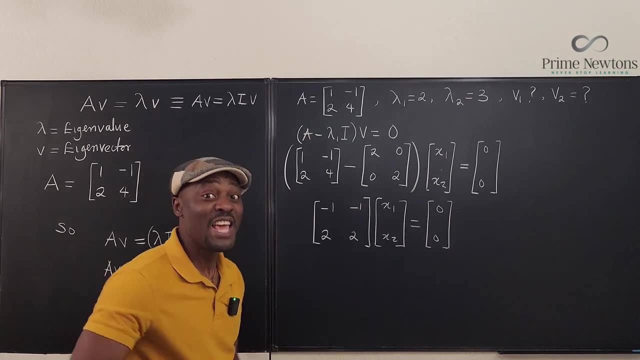 eigenvectors that when these things actually exist, you're going to get this. So if you really really want to get non-zero eigenvectors- that when these things actually exist and they're nice, this is the kind of answer you want. The two rows must give you the same exact thing If they're. 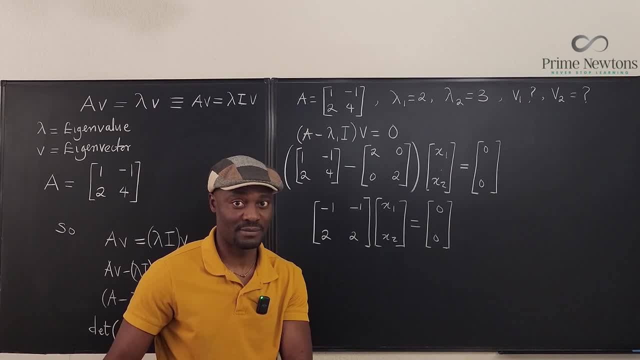 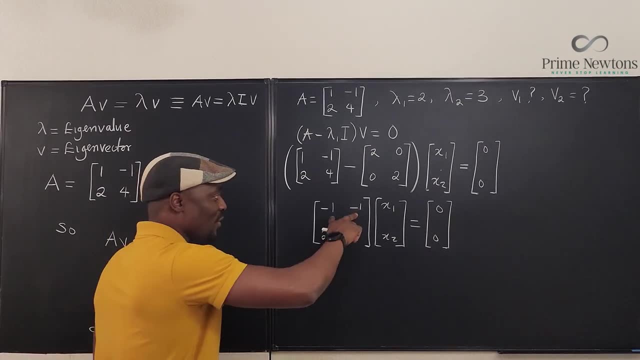 not the same. there's trouble lurking around. They have to be the same. Okay, So this is nice. Now what do you do? Use this row to multiply this. What do you get? Just take one of them, because both of them will give you the same result. Let's not waste time. 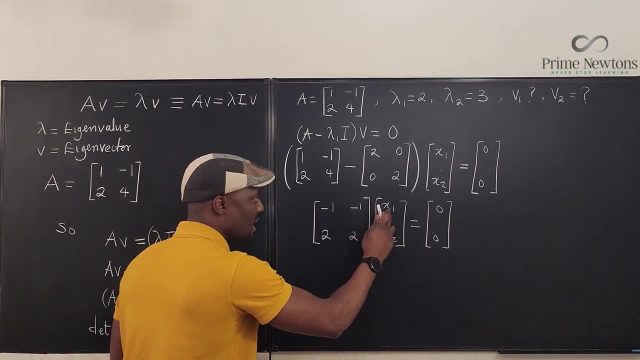 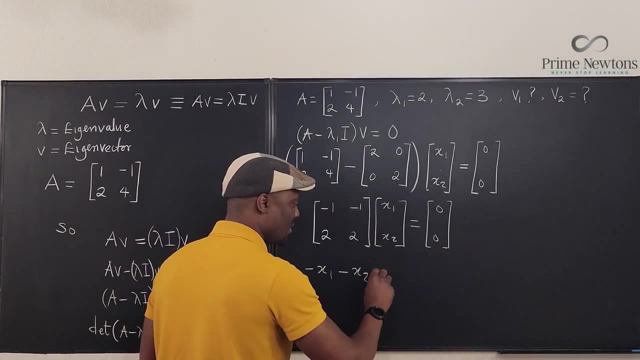 So you're going to have this. So what you have is: minus one times X1 is minus X1.. Minus one times X2 is minus X2, and the answer on the right-hand side is going to be equal to zero. So you've got an equation, Okay. So if you do the same thing here, you'll get the. 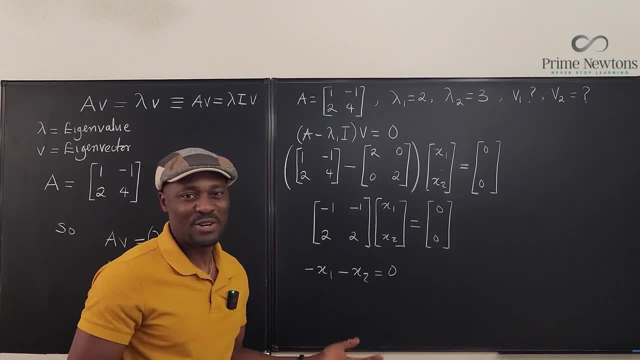 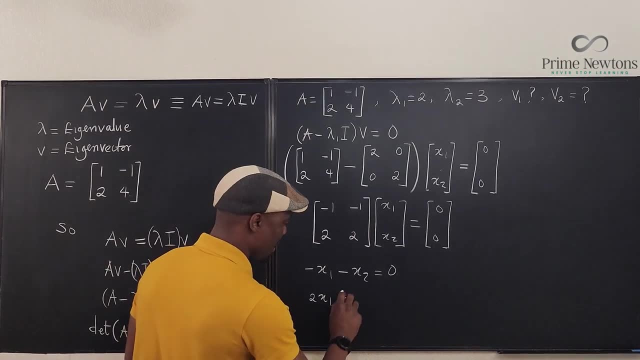 exact same thing, It's just this would be two, and you get rid of one of them and you still end up with this equation. Okay, let me just write it. So you end up with two X1 minus- sorry, plus two X2 equals zero. You see, If you do elimination, you will end up with 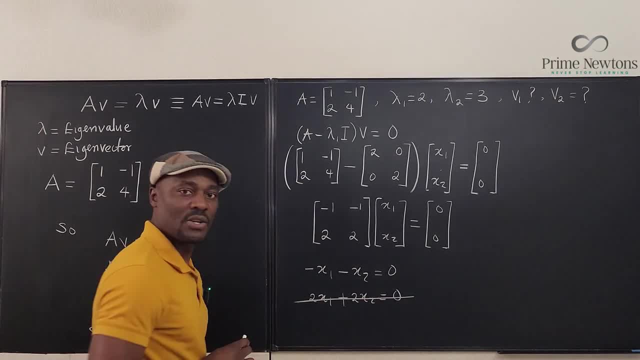 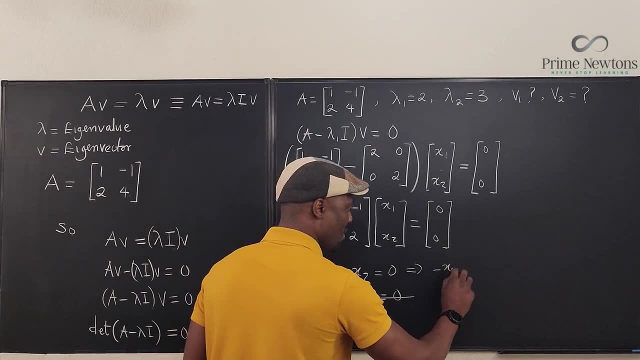 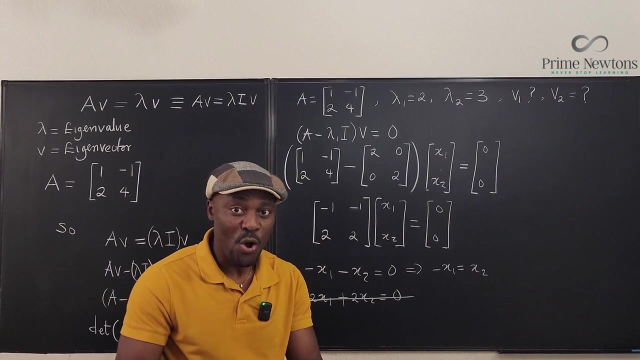 something like: so I'm just going to strike this out, Okay, Not necessary. And then what does this tell me? It means I can move this to the other side. This implies that negative X1 is equal to X2.. Now, this is my recommendation. What you're saying is: 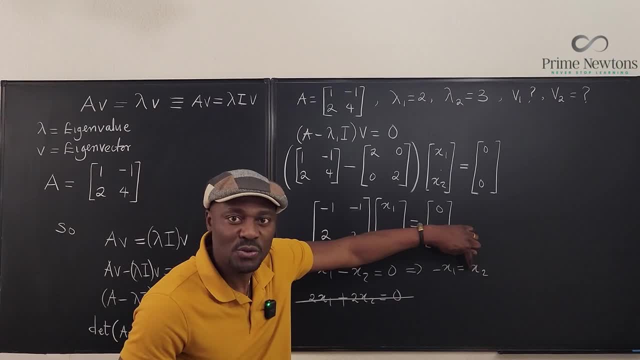 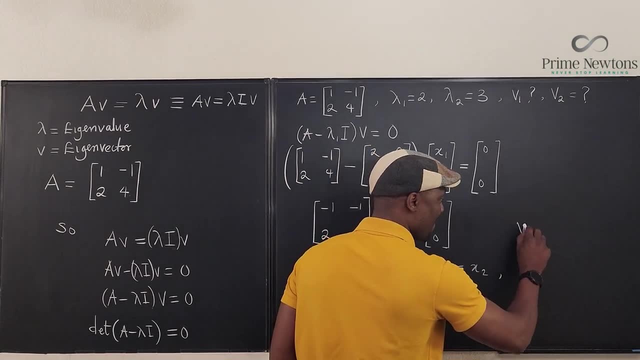 if I make this one my X1 one, what will X2 be? X2 will be minus one, So you can say that V one. Now, some professors are very strict with this. Okay, But this is what I will tell you. 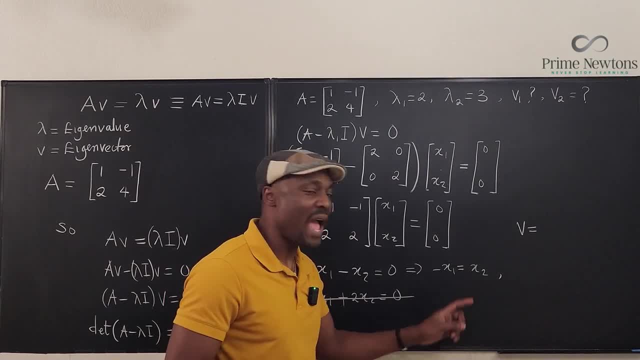 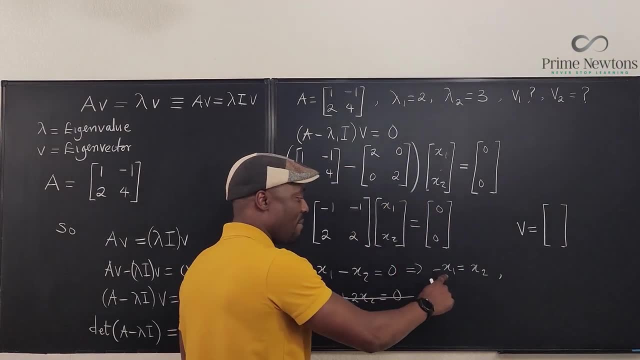 Be able to recognize your eigenvector. Just say: my eigenvector will be that vector that's standing like this: where, if my X1, if I make my X1 one, what will my X2 be? My X2 will be. 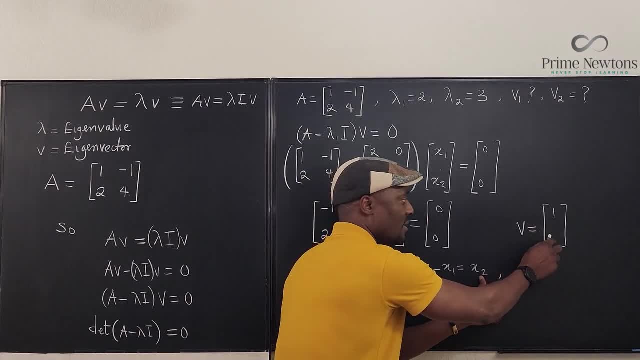 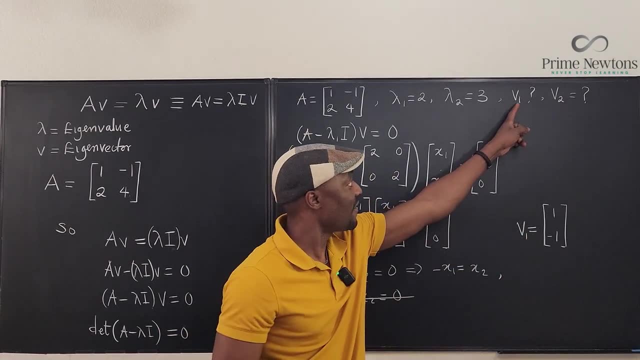 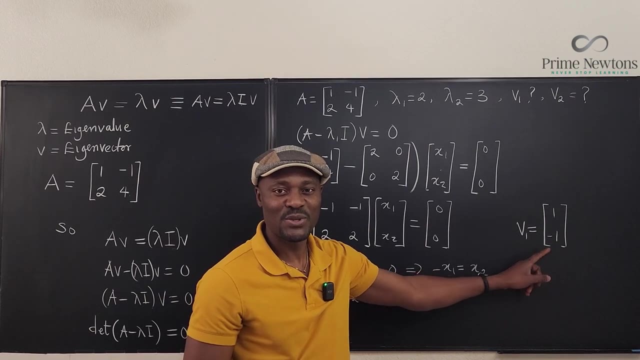 minus X1.. What is X1? One Minus X1 will be minus one. That is eigenvector one V one. This guy is this guy. You know what I'm going to leave the other one for you to do. 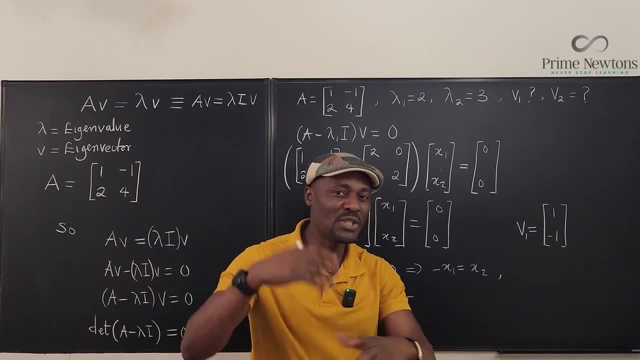 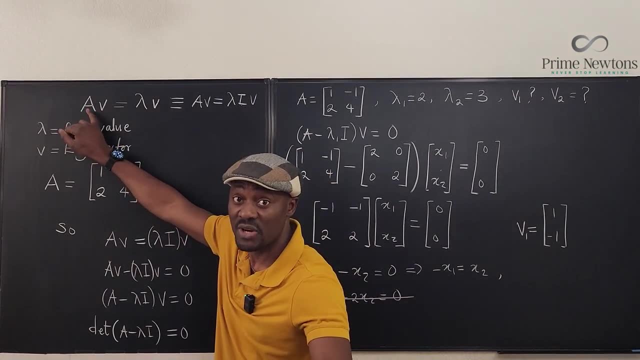 I'm just going to verify that this is true. Remember the original claim that we made? We made a claim that if you have an eigenvector and you multiply it from the left with a matrix, you don't have to use the matrix to multiply it. You can just multiply it by a. 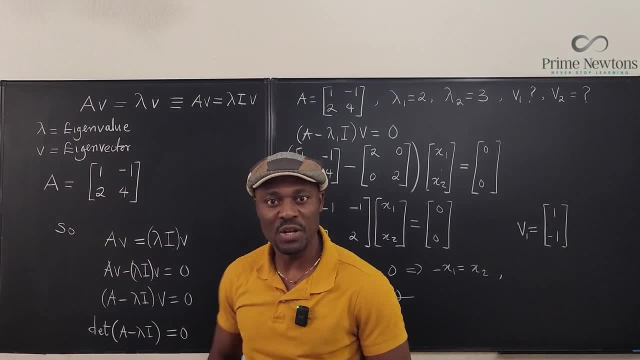 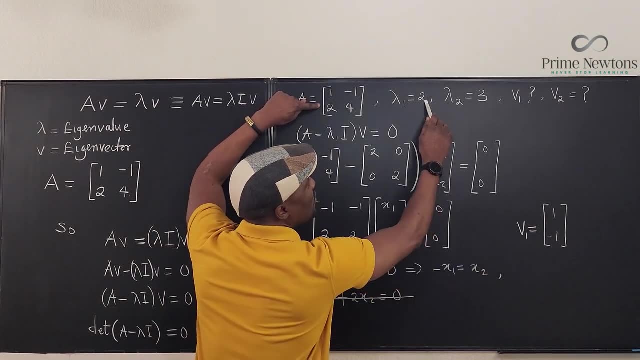 single number and the two sides will be the same. So we're going to test it, saying, instead of multiplying this eigenvector by this matrix, we're just going to multiply it by two and see if we're going to get the same answer. If that is true, I would let you also use this: 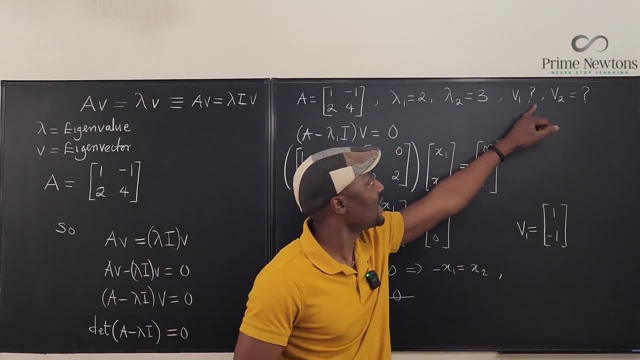 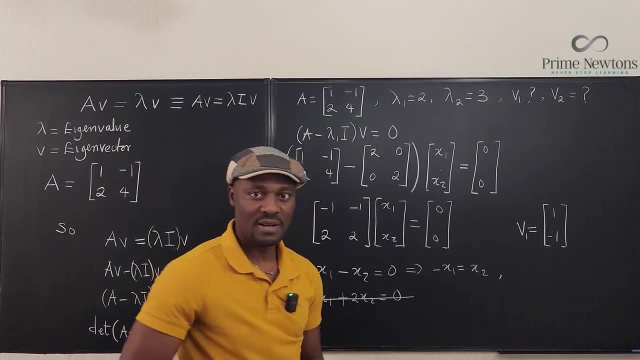 follow the same exact process and find the eigenvector for the second eigenvalue and then see if you're going to get your answer correctly. Let's verify this. Let's end the video, So I'm going to say A times V1,, which is: 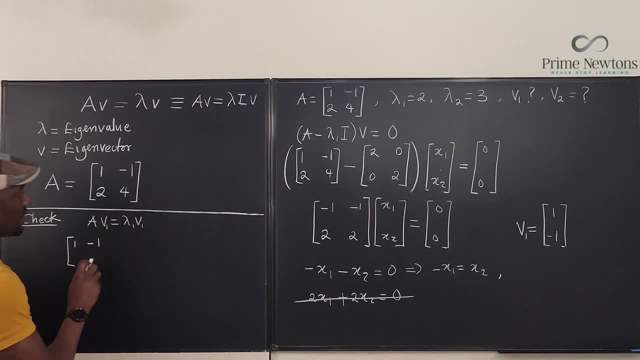 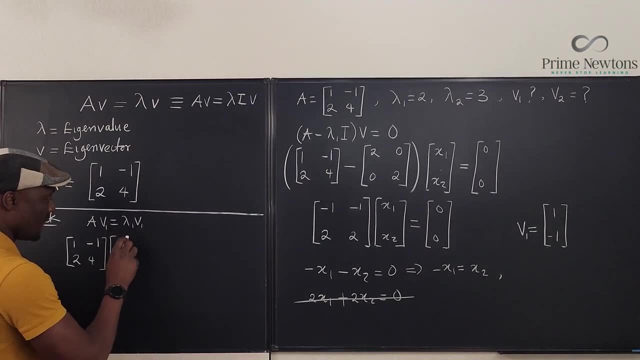 1 minus 1,, 2, 4, multiplied by V1, which is 1 times minus 1.. I'm going to say that this is equal to, with a question mark: what is my lambda 1? It's 2 times. what is V1?? V1 is 1 and minus 1.. 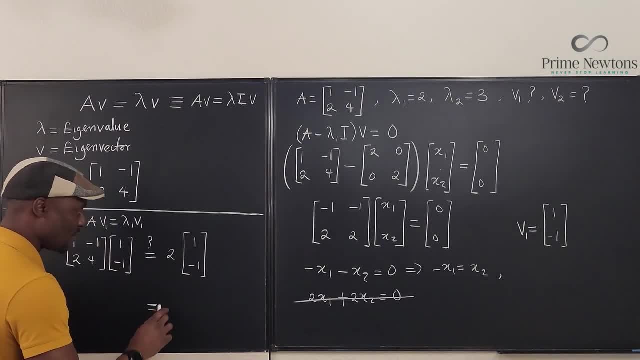 Well, let's see, The right-hand side is supposed to be 2 times 1 and 2 times minus 1.. So this should be 2 and minus 2.. Well, we better get the same answer on the left-hand side. Well, let's go.